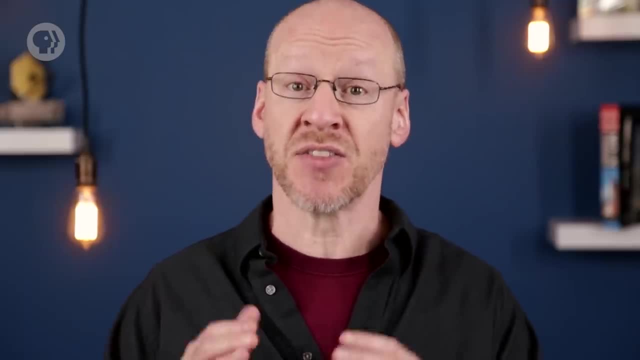 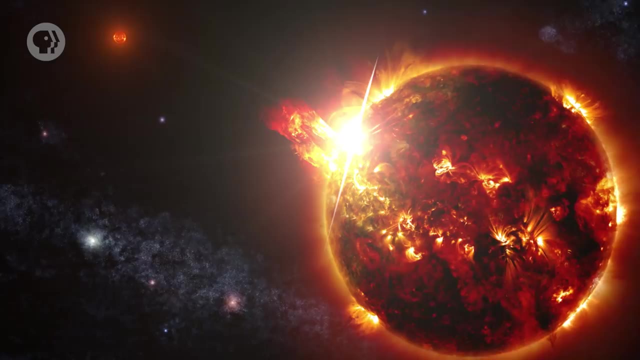 fuel in their cores more quickly. The lower mass a star is, the longer it lives. In the lowest-mass stars- cool red dwarfs- the rate is so slow they last a long long time. But there's more to it than that: They fuse hydrogen only in their very centers. 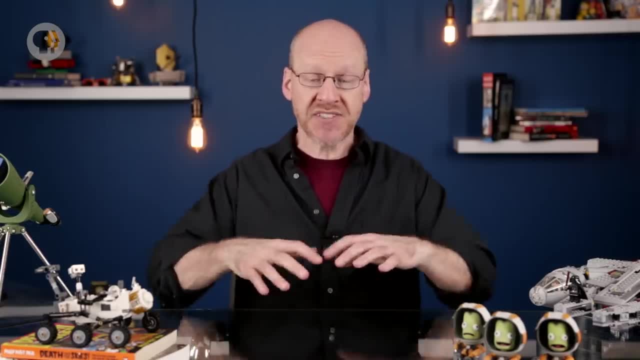 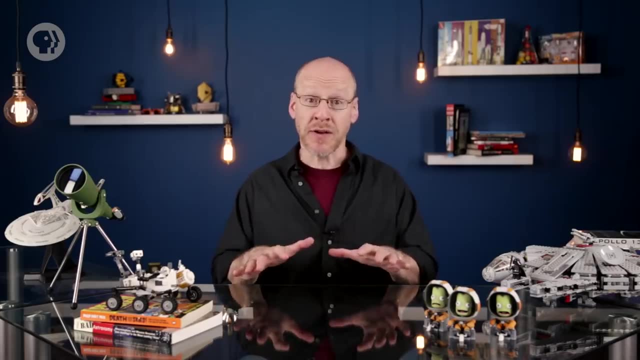 and their cores aren't very big Outside of this small region. the gas is convective, which means the hot stuff rises all the way to the surface, cools then falls back to the core. That's important because it means the entire star is available for fuel. Both 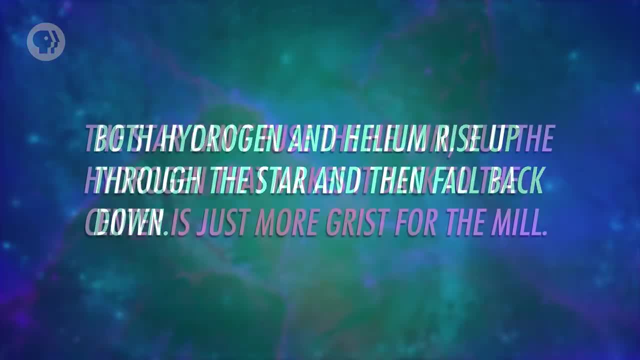 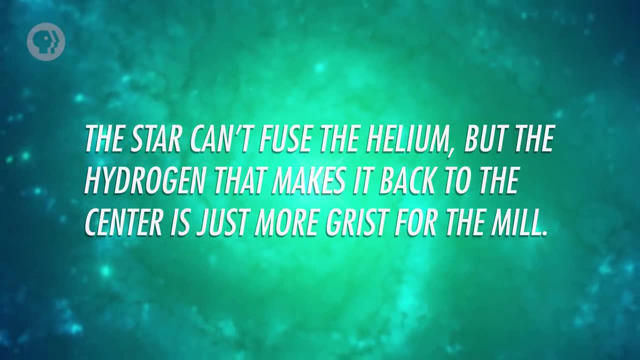 hydrogen and helium rise up through the star and then fall back down. The star can't fuse the helium, but the hydrogen that makes it back to the center is just more grist for the mill. Even after a long, long time, these stars can still shine as the hydrogen mixed. 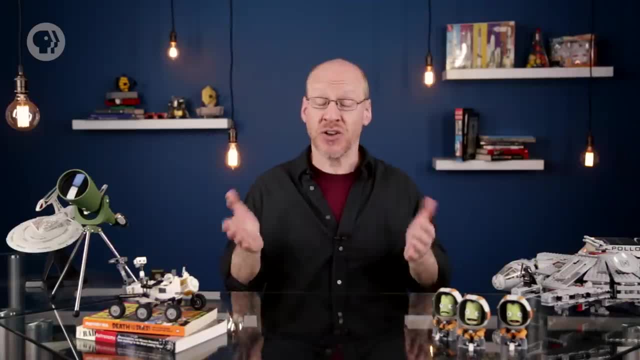 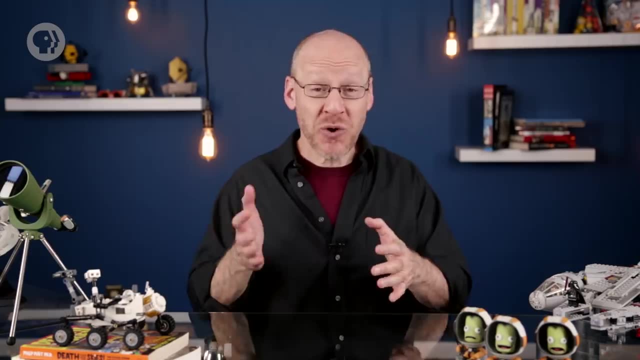 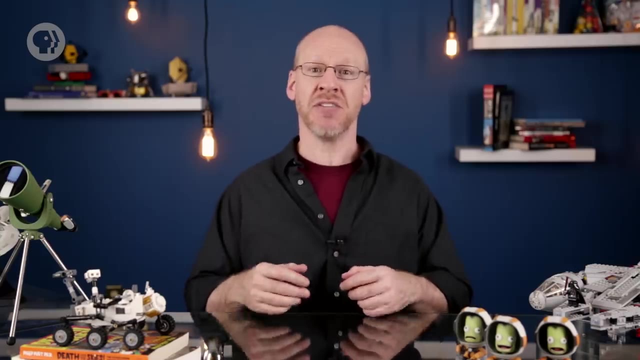 throughout the star, eventually makes it down to the center. So how long can a really low-mass red dwarf last? A trillion years, A trillion. The universe itself is less than 14 billion years old. so even the oldest red dwarf stars are basically infants. They're just barely getting a start in life and they'll look pretty much the same for the next oh, 990 billion years or so. Eventually, though, they do run out of fuel. When one does, the star itself will be nearly pure helium, plus whatever heavier elements it was born with, and fusion will cease It'll. 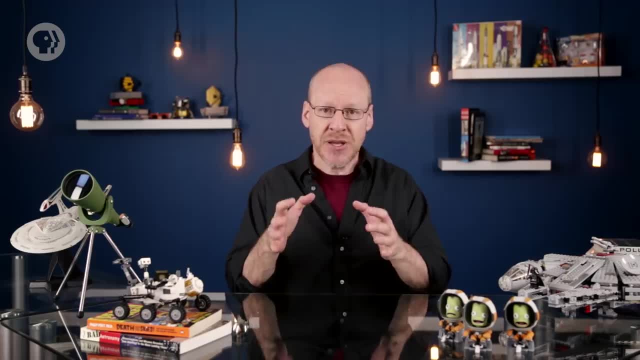 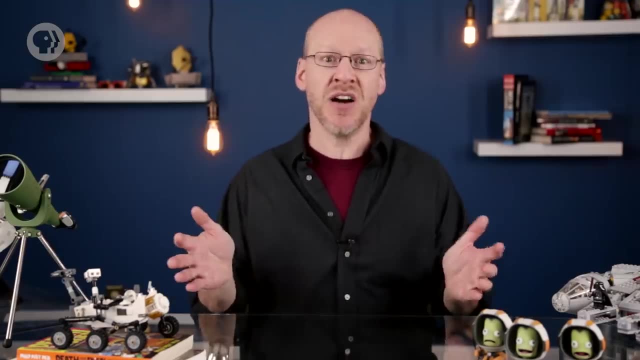 then cool, which will take many more billions of years. Finally, it'll be a cold, black dead star, And for them that'll be pretty much that, Or so we think. The universe is far too young for any of these red dwarfs to have run out. of fuel. yet That's true for stars at the lower end of the mass scale, up to roughly a third of the mass of the Sun. But stars with more mass than that, stars more like the Sun itself, work a little differently. Their cores are bigger and hotter and denser The different. 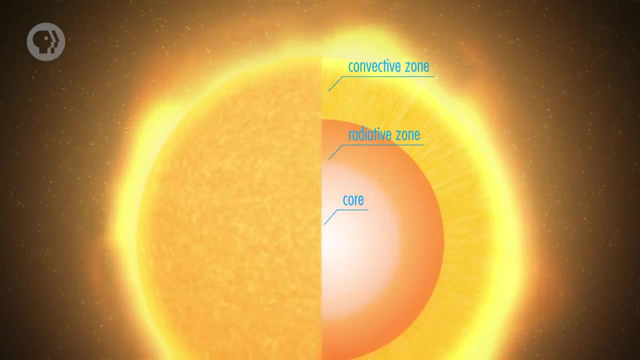 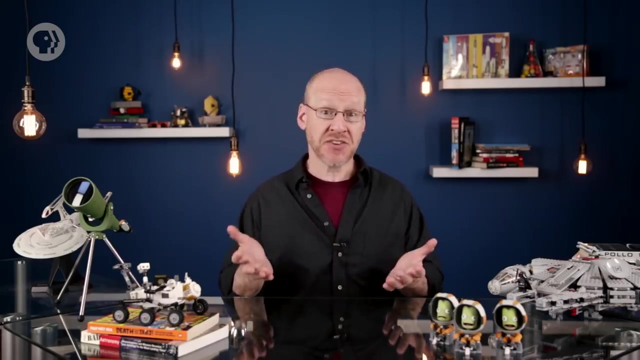 conditions inside them means the material in them doesn't convect. The hot stuff doesn't rise away from the core. What's in the core stays in the core. Outside the core there's a very deep and active convection zone, but that doesn't. interact with the material in the core itself. This means that not only do stars near the Sun's mass use up their fuel more quickly than red dwarfs, they have relatively less fuel to work with as well. Depending on their mass, their lives aren't nearly as long For the Sun that total lifespan is about. 12 billion years give or take. The Sun is nearly 5 billion years old now, so it's approaching middle age. Its life is similar to other stars of similar mass, so let's take a look into the far future. Will our Sun go gently into that good night? 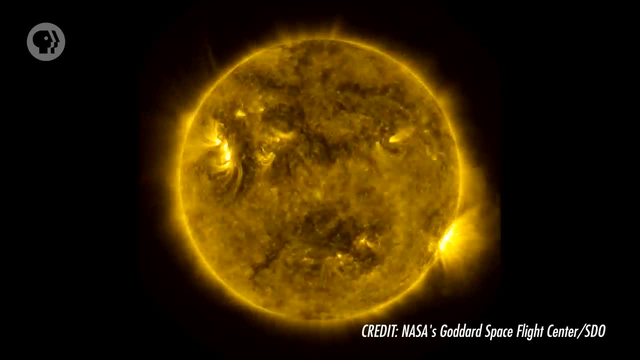 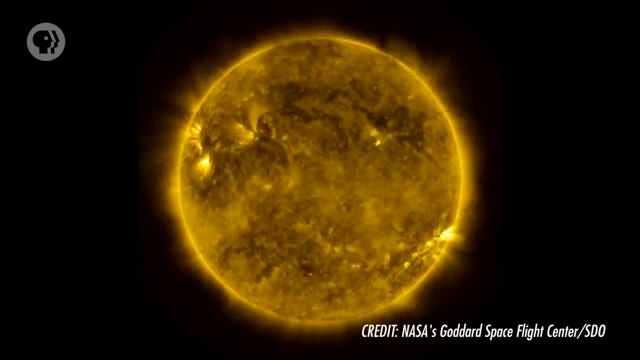 Ever since the Sun was born, it's been fusing hydrogen into helium in its core. The helium is trapped there, unable to be used as fuel, and it's building up in the core like ash in a fireplace. As it does, the density in the Sun's core slowly increases When you. 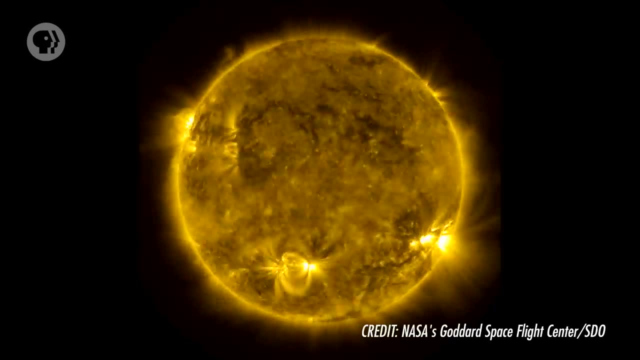 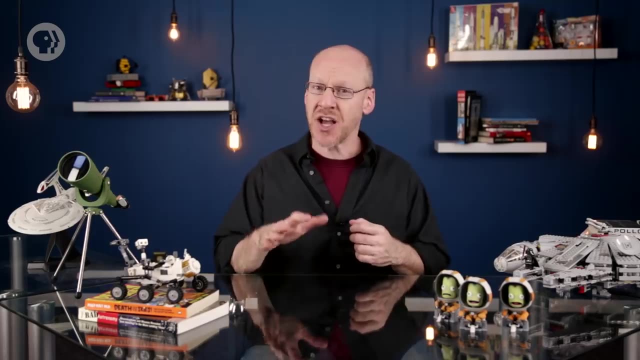 compress a gas, it heats up. That means every day the Sun's core gets a wee bit hotter. That extra heat works its way out through our star, heating up the outer layers too. A hotter gas shines more brightly, so the Sun has been steadily increasing in brightness too. It's an incredibly slow but inexorable process. The Sun's increased in luminosity by about 40% since it was born And it's not done. Helium is still building up in its core and eventually it'll run out of hydrogen to fuse Without fuel fusion in the core. 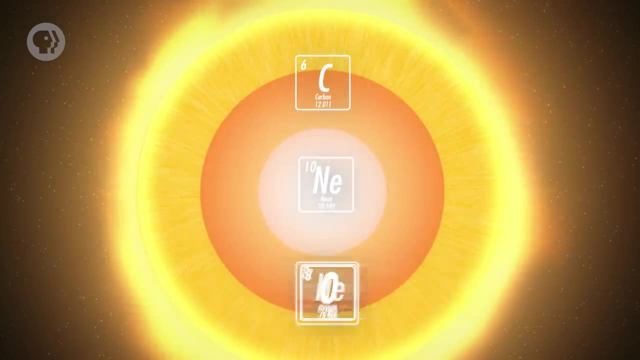 will stop. Helium can be fused into carbon and a little bit of oxygen and neon, but it has to be incredibly hot to do so and the Sun's core won't be anywhere near those conditions. Still, half the Sun's mass is bearing down on the core. So even though fusion stops, the core will continue to contract. 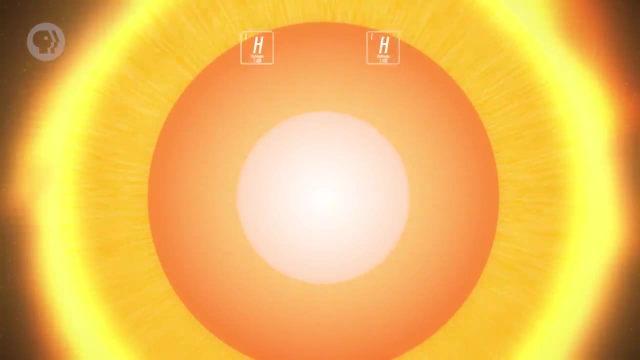 and heat up. It'll get so hot that the temperature outside the core will get to hydrogen fusion temperatures, Like igniting a match by holding it near a flame. the hydrogen outside the core will start to fuse. That'll occur in a shell surrounding the core, adding its heat. to the outer layers of the Sun as well. When you heat a gas, it expands The Sun's outer layers will do just that, and our star will grow to well over twice its current size. Astronomers call a star like this a subjunction. Not only will it grow, but its color will change. The Sun will be giving off more total energy than it does now, but its surface area will increase so much that the amount of energy radiated per square centimeter will go down. There'll just be a lot more square centimeters. This means, ironically, that the surface will actually cool. The Sun's temperature will go down Cooler stars are red, and so the Sun will be too, But the core still isn't done. The details are complicated, but the core continues to. 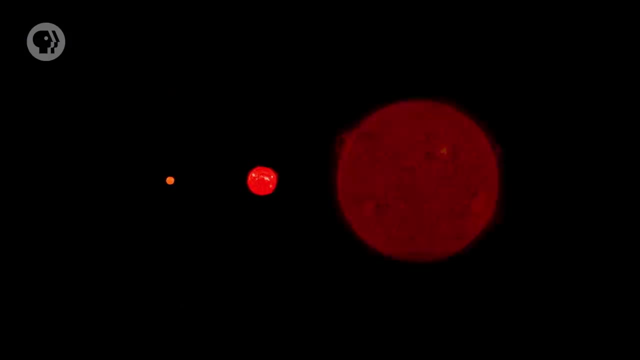 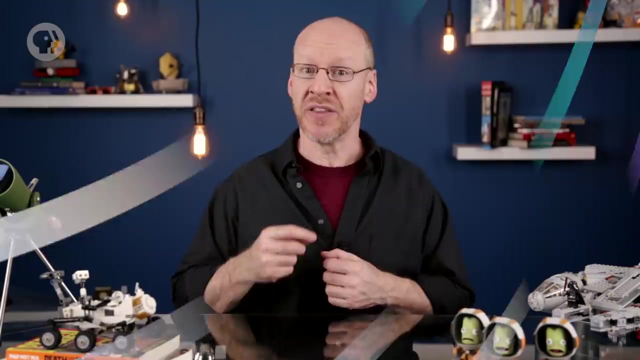 contract and heat up. It gets so hot that the outer layers swell even more and the Sun can blow it up to a fantastic 10 to 150 times its present size. It will then be a red giant. Red giants are fantastically bright because of all the energy percolating up from their interiors coupled with their enormous size. When it turns into a red giant, the Sun will increase its luminosity by an incredible 2,000 times. That huge increase in luminosity does more than just make the Sun bright, though. As a red giant, the Sun will be so swollen that the gravity at its surface will drop. substantially from what it is now. The force of gravity holding it down is weak, but the force from all that light blasting out from below is strong, easily overpowering gravity. Material on the surface will get blown off like a leaf in a hurricane. 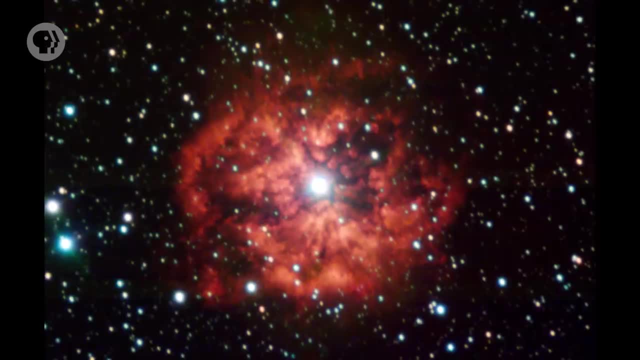 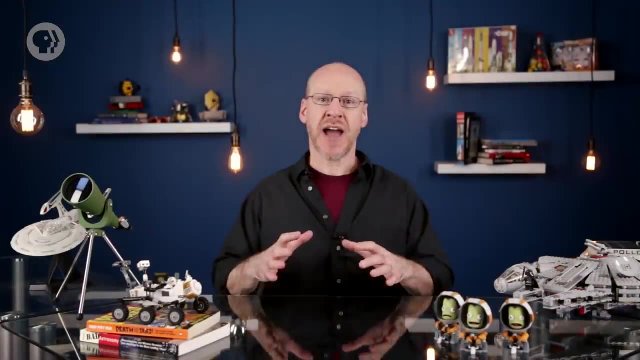 Think of it as a super solar wind. That means the Sun will shed mass a lot faster than it does now. While it's a red giant, it'll lose fully a third of its mass At some point. the core contracts and heats up so much that the conditions will finally be primed for helium fusion. Suddenly, helium is converted into carbon, releasing a lot of energy. In a weird twist, due to a lot of very complicated physics, the core itself winds up expanding, absorbing most of that energy. In the end, less energy is pumped into the outer layers, so the Sun's outer layers contract, The Sun shrinks, The outer layers get dense again, which warms them up a bit, and the Sun turns from red to orange. It's still pretty big, more than 10 times its current day size. 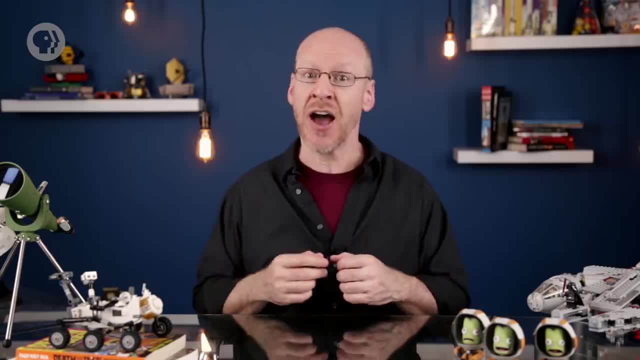 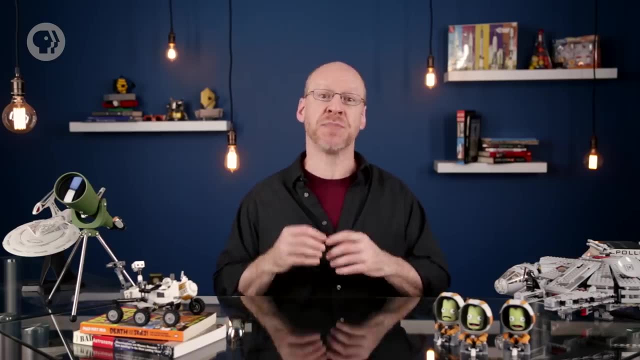 And it puts out 20 to 50 times as much energy as it does now. But then we see a sort of reboot of what's happened in the core before. This time, though helium is fusing in the core and the carbon is building up like ash. 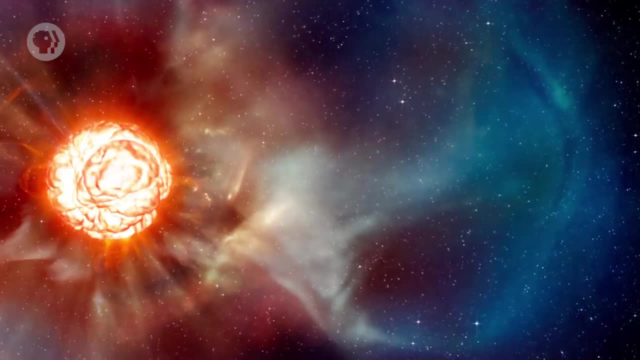 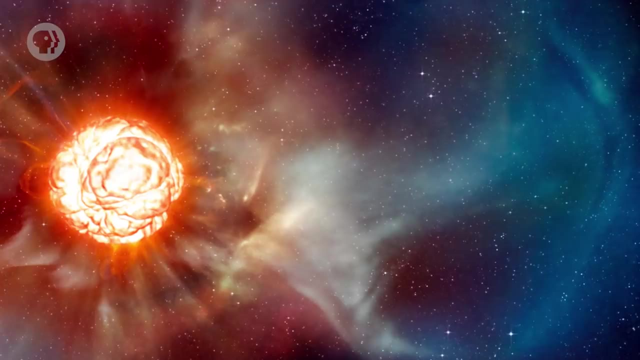 Once again the core starts to contract and heat up. This dumps more energy into the outer layers. they expand and cool and the Sun turns into a red giant again. This time it's even brighter and bigger and loses even more mass, shedding over half. 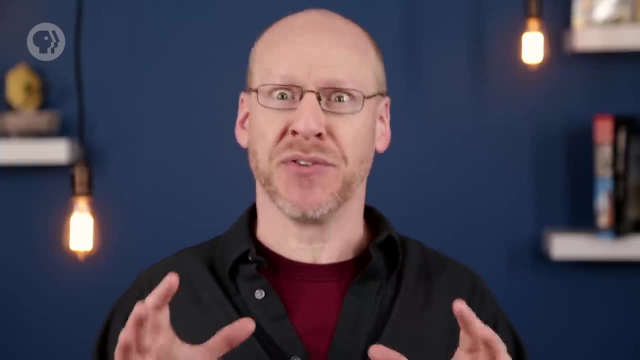 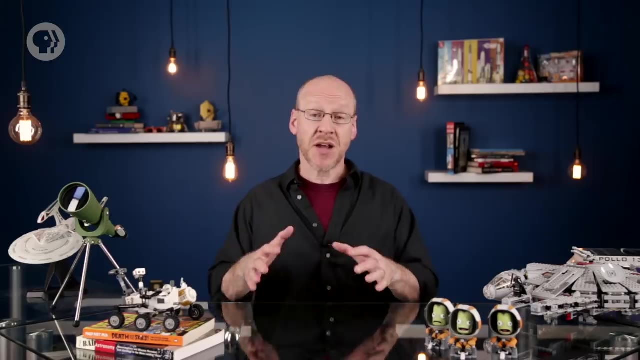 of what's left. In the meantime, helium fusion isn't very stable, To say the least. it swings wildly, increasing and decreasing its rate by huge amounts on very short timescales. The Sun will probably undergo a series of tremendous paroxysms, epic eruptions as the 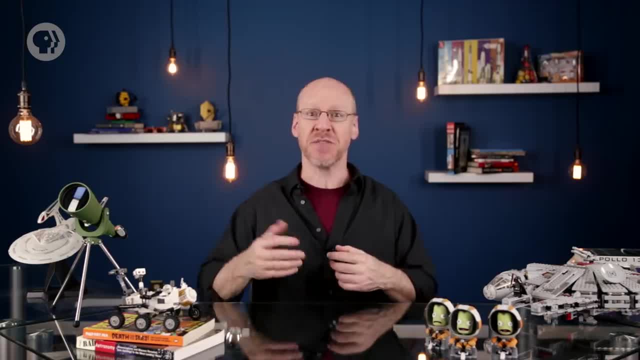 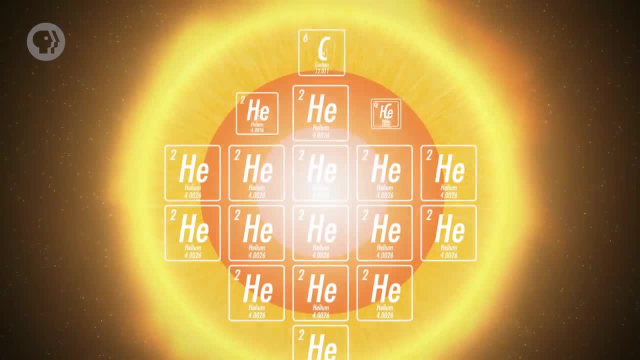 helium fusion spikes, creating huge surges in energy production, It'll lose even more mass each time. Finally, though, we approach the endgame. The Sun doesn't have enough mass to squeeze carbon atoms, enough to fuse them. They build up in the core until there's no more helium and fusion stops. 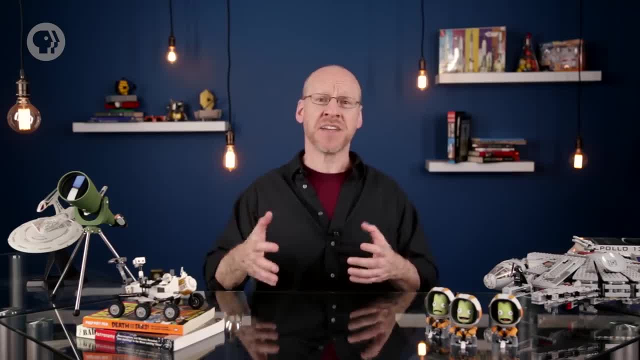 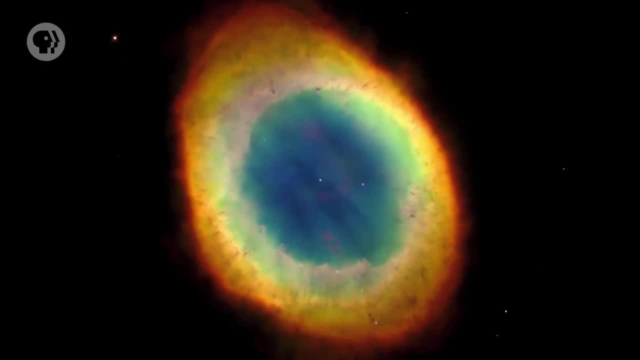 On top of that… Well, there's nothing on top of that. By this time, the Sun will have literally blown off all its outer layers. It's essentially a naked core, a hot, intensely bright, super-compact ball, not much bigger. 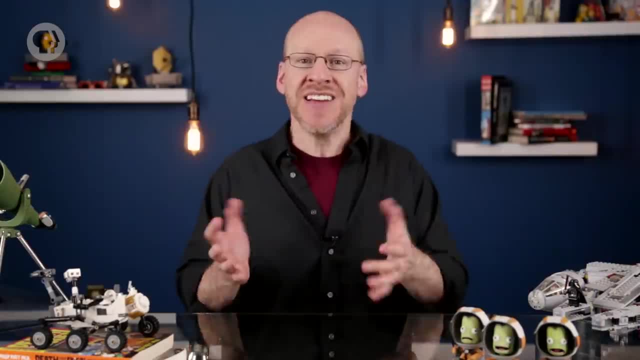 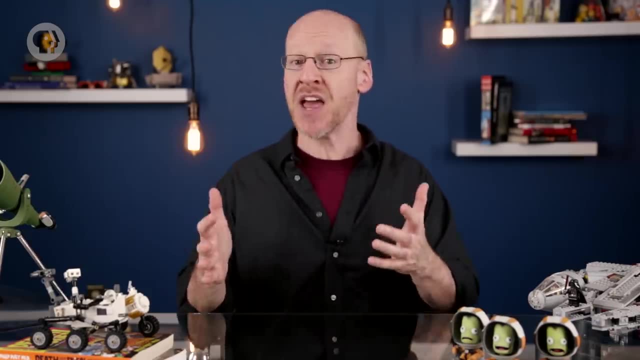 than Earth. We call this a white dwarf. Its fate is sealed. It can't generate energy, so it'll cool and fade over the next few tens of billions of years. At that point we can safely say the Sun is dead. But that's not always the case for all stars. 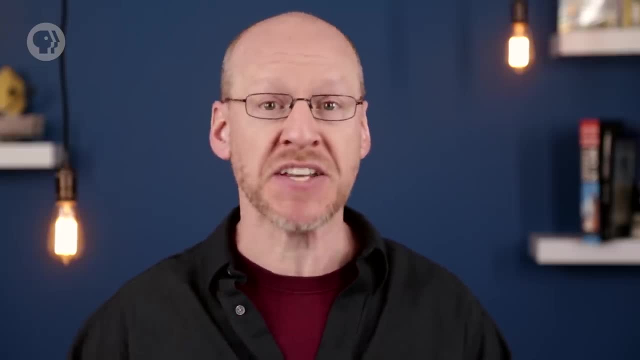 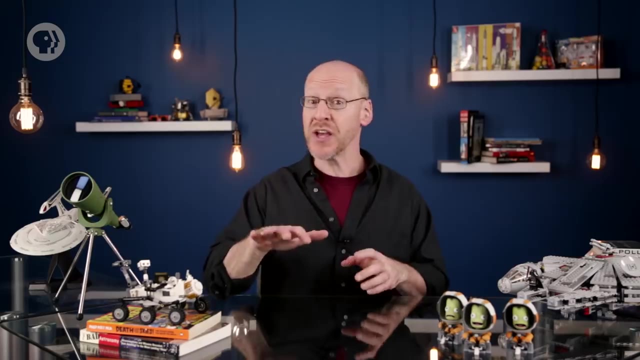 Some with more mass than the Sun, still go through another phase before it's dead. They form what are called planetary nebulae, And these are so amazing and beautiful that they rate their own episode, which, along with more fun stuff about white dwarfs, we'll get to next time. 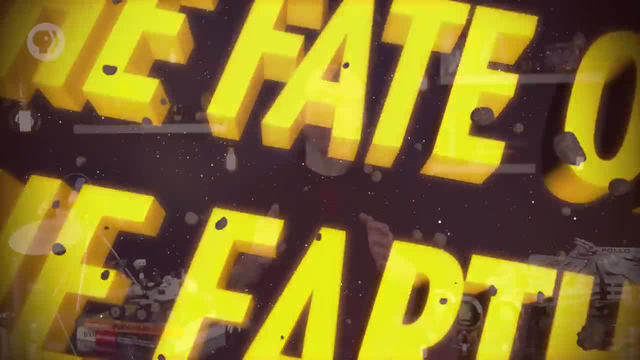 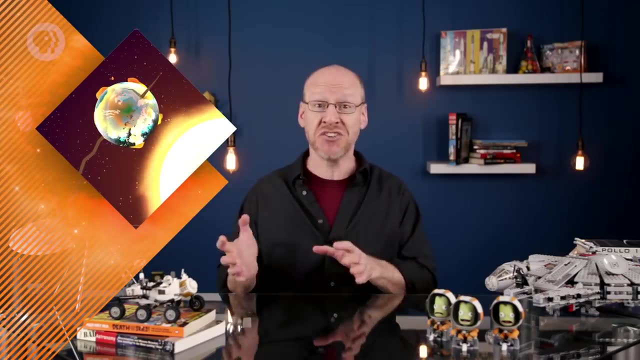 So that's it for the Sun. But what about us? Of course, the Earth won't fare very well during all this. It'll get cooked before the Sun even becomes a sub-giant, and by the time the Sun is a red giant, we'll be good and fried. 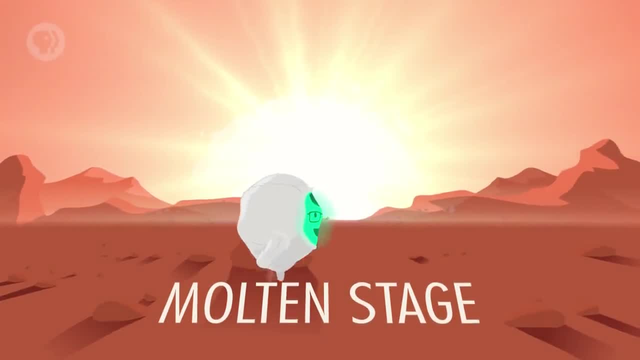 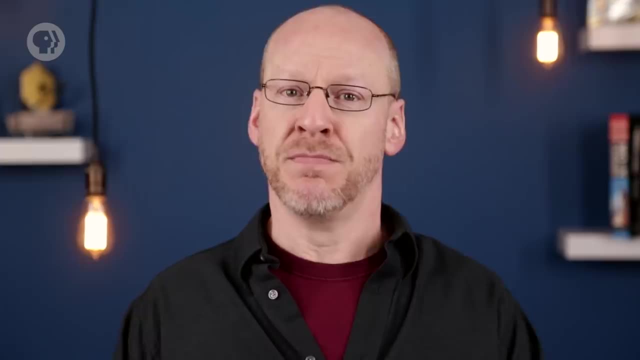 The average temperature on our planet will be so high that it'll melt rocks and in a sense, it'll look much like it once did. But that's not all. It once did so many billions of years before when it first formed a molten ball of rock. 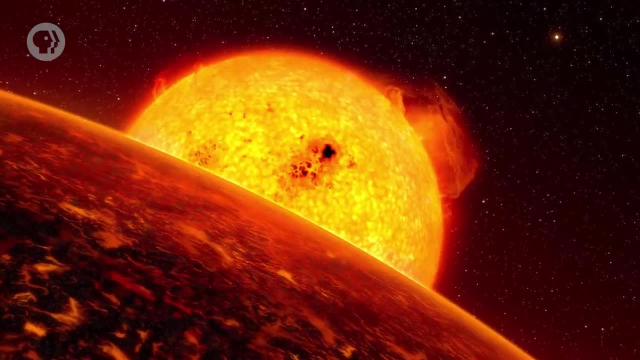 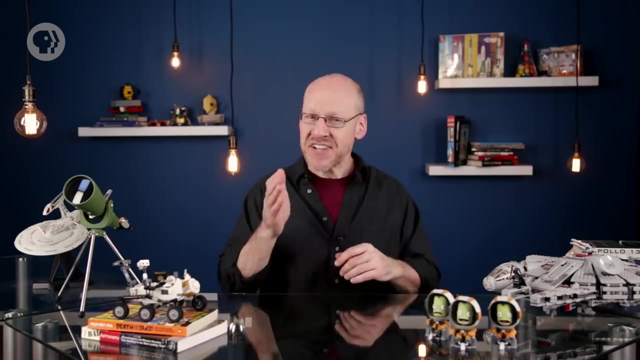 But it gets worse. When the Sun expands, it'll reach a radius very close to the size of the Earth's orbit. now, Does that mean our planet itself will be consumed by the Sun? Maybe not. As the Sun expands, remember, it loses mass. That means its gravitational pull will weaken and Earth will move out from the Sun into a bigger orbit. If things work out right for us, the Earth will back off faster than the Sun expands and we'll avoid finding out what it's doing. That's what it's like to be inside a star. Due to a quirk of physics, if the Sun loses more than half its mass, its gravity will decrease so much the planets will no longer be gravitationally bound to it, and they'll. be flung into interstellar space. I'm not sure that's any better for us. Either way, the Earth will have been long dead and hopefully humanity will have figured out the trick to interstellar travel by that time. All those Earth-like exoplanets around younger stars will look pretty nice in a billion years. or two. Mind you, this isn't happening any time soon. The Sun won't become a subject. We'll have to wait and see. The Sun will be a giant until it's nearly 11 billion years old, over 6 billion years. from now. The first red giant stage happens when it's over 11.5 billion years old, and the second stage a half billion years later. This is a long, long time coming. If the Sun had more mass, it could avoid this fate. A star with about eight times the Sun's mass can. It has enough mass to squeeze those carbon nuclei hard enough to fuse them together. Those high-mass stars have a much different and far more explosive fate than lower-mass stars like the Sun.